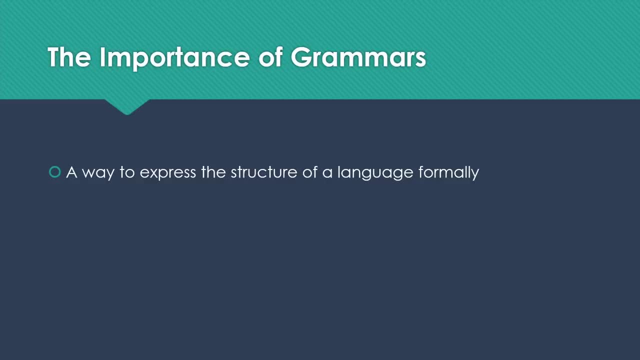 since you're listening to this in English, you understand a little bit about how the English language works. As we think about programming languages, a key thing that grammars do is they help the person creating the language, clarify and communicate the structure of the language to. 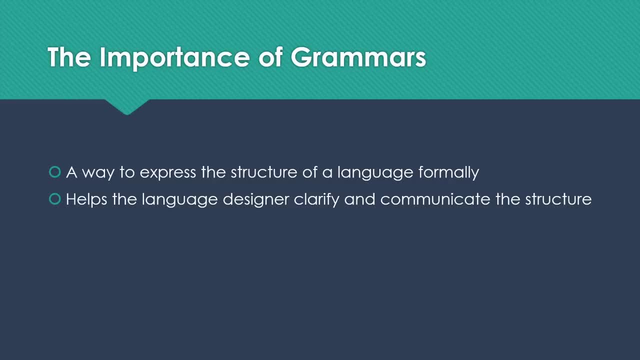 others. The grammar for a language can also help us understand it. As we're learning or trying to more deeply understand a language, it can be useful to look at the grammar for the language to see how it's supposed to work, So we know the rules. Finally, if we're tasked with implementing, 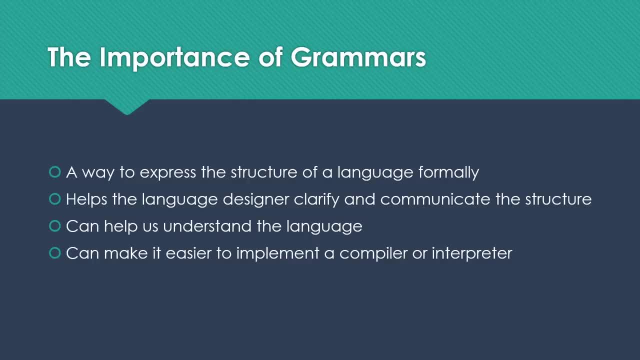 a compiler or an interpreter for a language. the grammar is a key piece of that, And often we have a piece of the language that we're trying to understand, So we can see how it's supposed to work. And we can see how it's supposed to work. And we can see how it's supposed to work And we can. 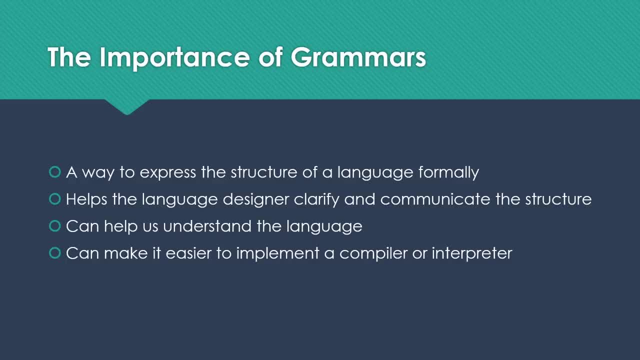 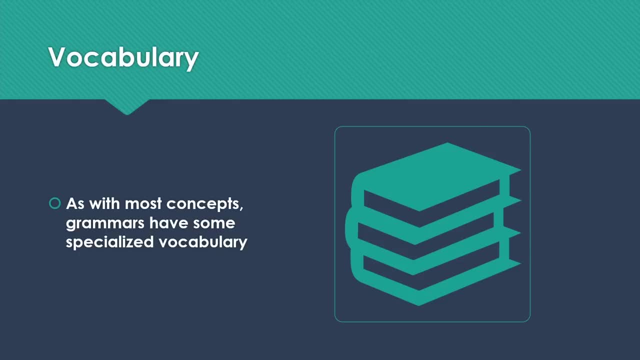 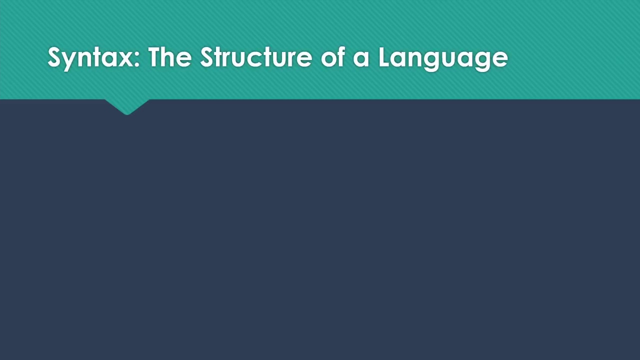 understand what that is. So this is kind of defines the airline of the compiler or the interpreter. that looks almost exactly like a grammar for the language. Before we get into actually looking at what produced now reformed gram exercise looks like, we look at here a little more vocabulary. there are some things that we need to understand some. 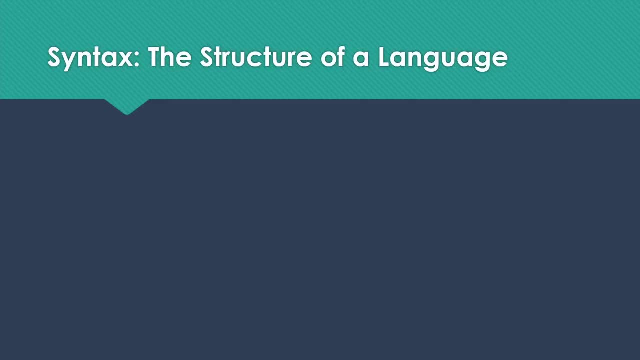 terminology that we need to be clear on for grammars. First of all, syntax, So a syntax of a. so let me give you a few English examples to help you get at this idea. so here I have a simple sentence: the girl ate the pasta. this is a correct sentence with correct structure. then I have 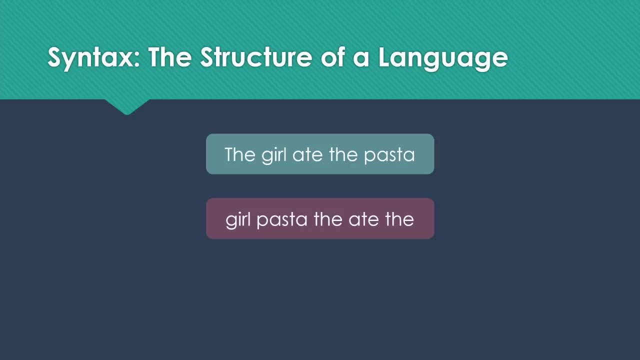 something with the same words in it, but girl pasta the ate the is not syntactically correct. there is no structure of English that allows that to be a sentence. we can also see the effects of syntax in this next one, which uses the same words again: the pasta ate the girl. same words. 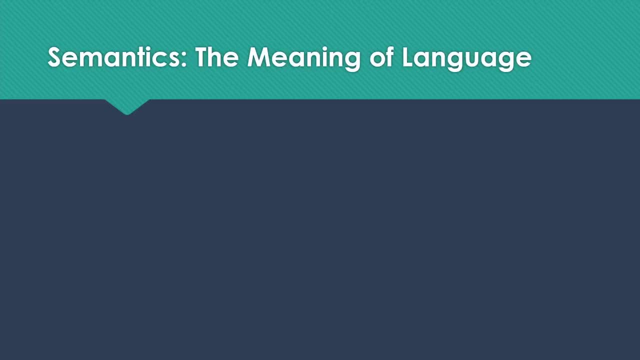 slightly different structure. semantics is another aspect of language which is really about the meaning of the language. we're not going to talk a whole lot about semantics in this video, but I do want you to have a look at some of the other semantics that we've talked about in this video. 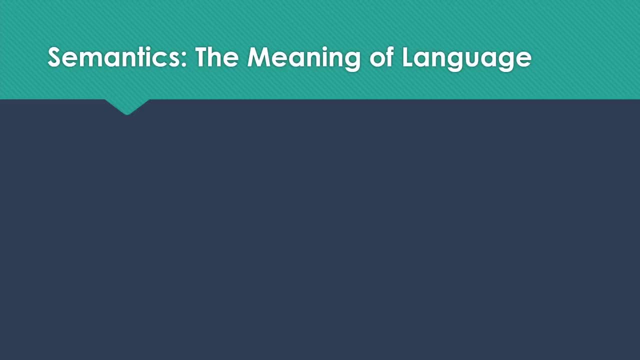 some understanding of what it is and sort of see how it's going to connect to our syntax. so we have wrong syntax, in a programming language at least, we have no meaning. so if your syntax is wrong, the compiler or interpreter can't do anything with what you've written and no meaning will result if the syntax is wrong enough. that's also true of 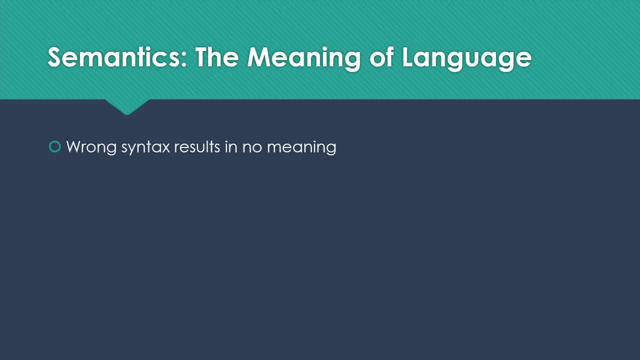 natural language. so certainly our second example on the previous slide had no meaning in a natural language. we have no meaning in a natural language. we have no meaning in a natural language. correct syntax can sometimes result in something meaningless. so a standard example of that: his colorless green ideas sleep furiously. that's syntactically completely correct, perfectly good. 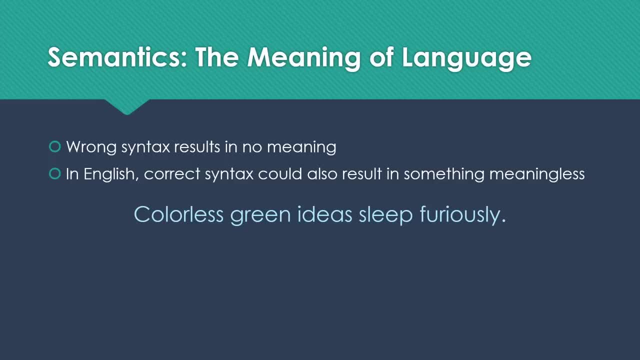 English sentence, in terms of its structure, has no meaning. one of the things that we try very hard to do is to make sure this can't happen. in a program that if we have a syntactically correct sentence, there is a meaning, the syntax is correct. in a program that if we have a syntactically correct sentence, there is a meaning, the 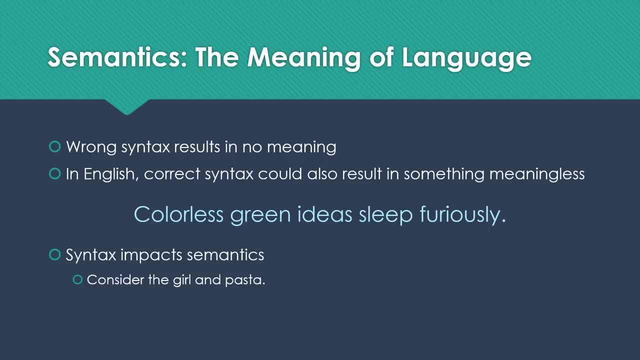 the computer can execute. one thing I want you to be very aware of, and one thing that we will focus on in the next video, is that syntax impacts semantics. so if we think about the girl and the pasta, how the syntax was done- whether the girl was the subject of the sentence or the object of the sentence- made a huge difference. 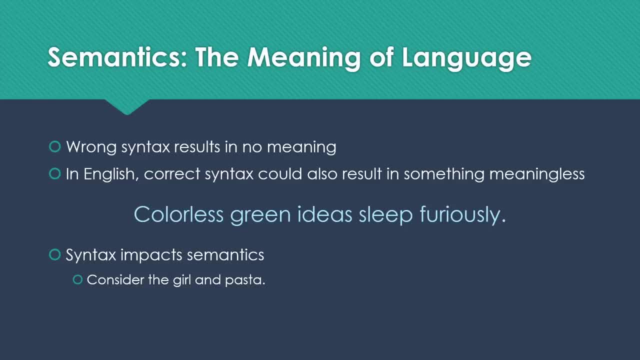 to the meaning of the sentence, and that's going to be true sometimes for a the sentence, and that's going to be true sometimes for a the sentence, and that's going to be true sometimes for a programming languages and their grammars as well. another thing we need 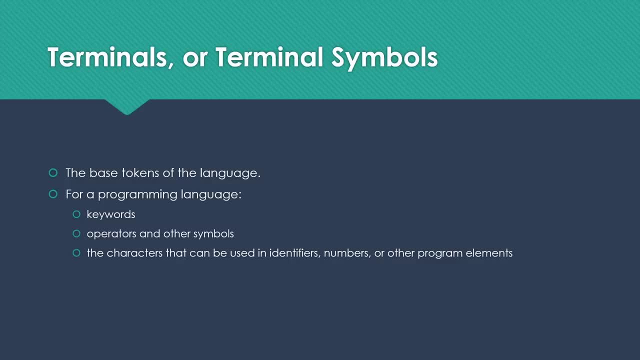 to understand is what terminals or terminal symbols are in a language. so these are the base tokens of the language. for a programming language that might be keywords, operators and other symbols. so plus minus your asterisk for times, parentheses, curly braces and so on, and then the characters that can be used. 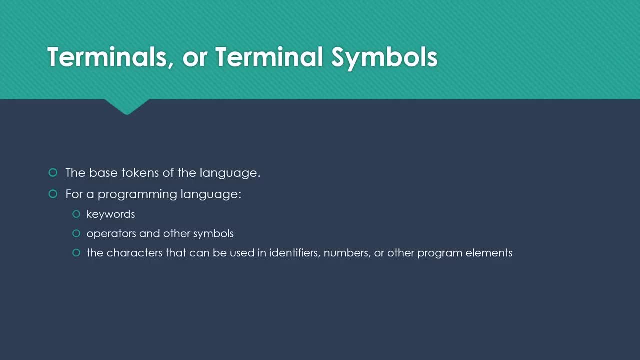 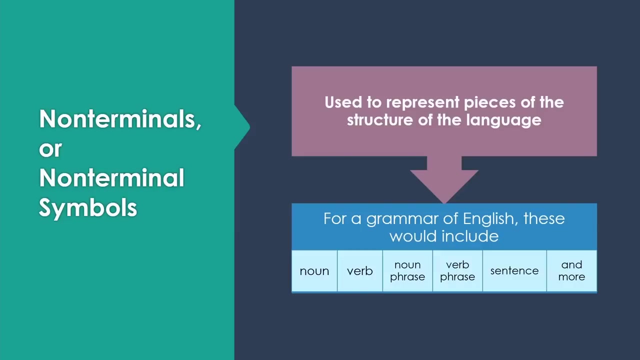 in identifiers, in numbers or other program elements. these are the things that make up the actual program we're going to read. non-terminals, or non-terminal symbols, are used to represent pieces of the structure. for a grammar of English, these would include things like noun, verb noun. 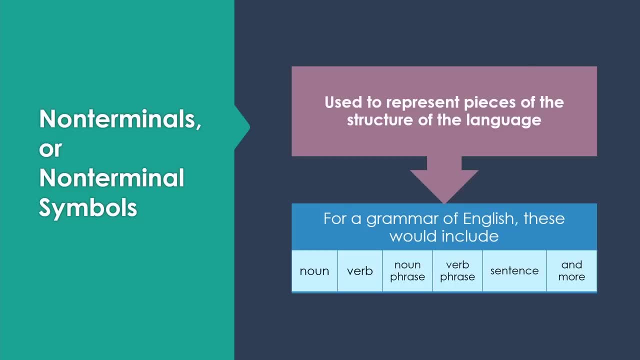 phrase, verb phrase, sentence. for a programming language they might include things like statement or condition or subroutine. they basically identify pieces of the syntax that it makes sense to work with, but notice they don't appear in the actual program. these are labels for parts of the program that make sense as part of the structure. and then, finally, we have productions. 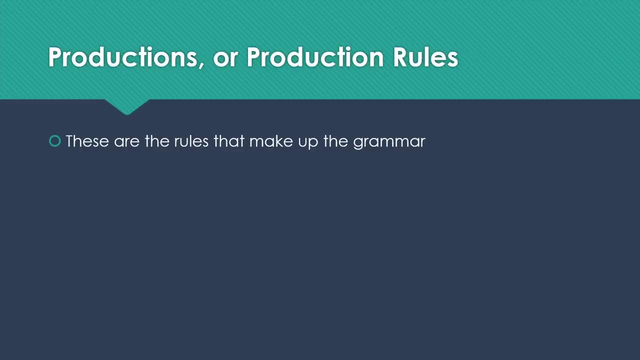 or production rules. these are the rules that make up the grammar. the things that connect are non-terminals and are terminals to define what the language looks like. so each rule is going to translate a non-terminal to a sequence of one or more non-terminals or terminals. 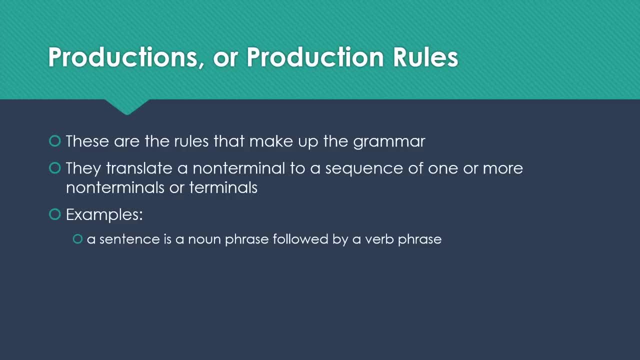 so some examples of that a sentence might be a noun phrase followed by a verb phrase, and in fact in English usually is a verb phrase, is typically a verb, or a verb followed by a noun phrase. then a verb would be one of a list of words, things like saw, liked, ate, visited, loved and. 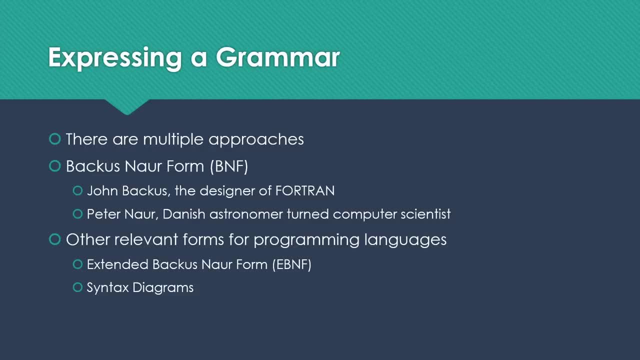 so on. now that we have an idea of what goes into a grammar and what we're talking about, I want to talk a little bit about expressing a grammar. there are lots of ways to do this. three key ways are used for programming today. we're going to focus on backus now: reform or BNF. 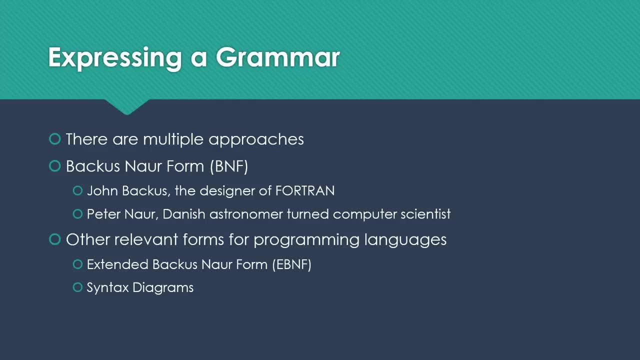 which is the simplest of our approaches. in many ways, it was created by John Bacchus, who also designed Fortran, and Peter Naur, so Bacchus Naur simply are the two people who created it. there are two other major forms that get used for programming languages extended: Bacchus Naur. 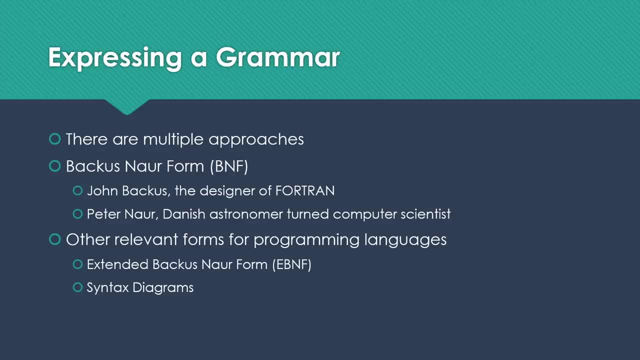 form, or EBNF, which adds some other elements to the Bacchus Naur form in order to allow it to be more, more compact but a little bit more complex, and then syntax diagrams, which are really graphs of the syntax of a language. this can be easier to understand in some ways than BNF or EBNF, but it 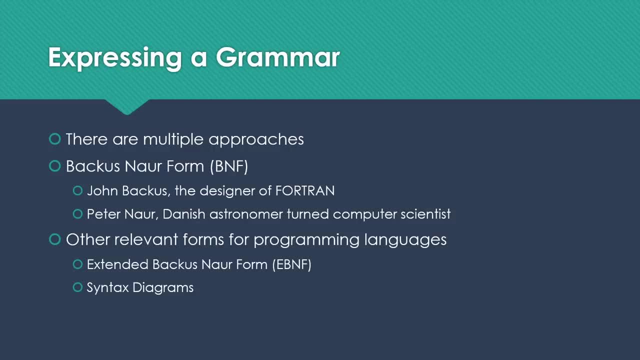 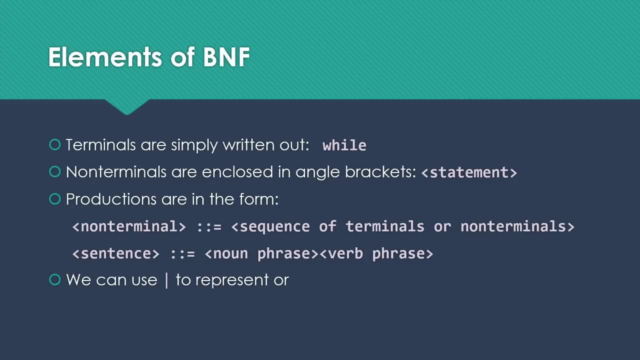 tends to be less compact and it is much harder to turn into a program or to work with programmatically. first of all, we need terminals. those are simply going to be written out. so while we need a while, that keyword we're just going to write, while non-terminals are going to be enclosed in angle. 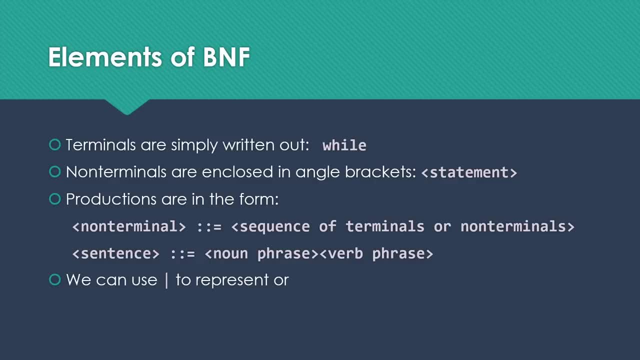 brackets so we can distinguish them from the terminals. then productions are going to be in the form some non-terminal, then colon, colon equals, and then some sequence of terminals or non-terminals, including that sometimes that colon, colon equals symbol is written a little bit differently. you might see it with just one colon, you might see it with a colon followed by a hyphen or dash. 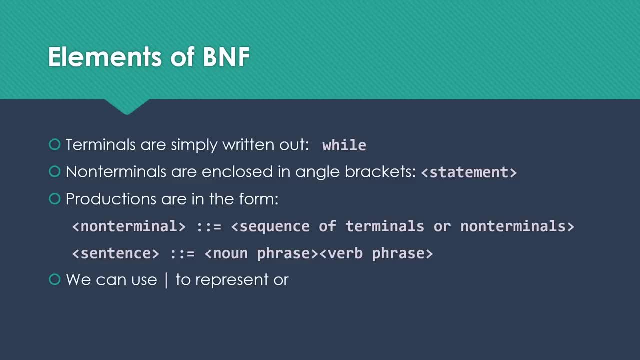 this, however, is the most common version of the syntax. here's an example: sentence goes to noun phrase, followed by verb phrase, where noun phrase and verb phrase are also non-terminals. the only other thing we have to worry about in terms of what the elements BNF are is that we can use the pipe symbol or the vertical bar to represent or, And that's all there. 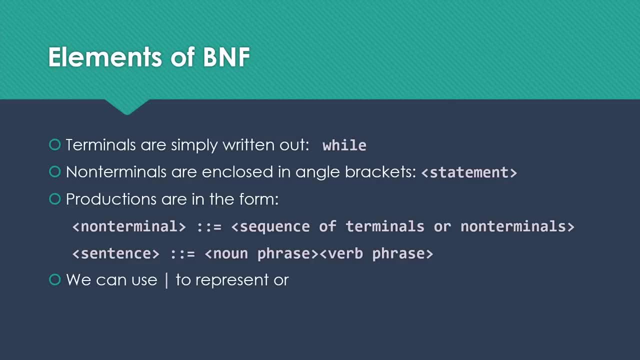 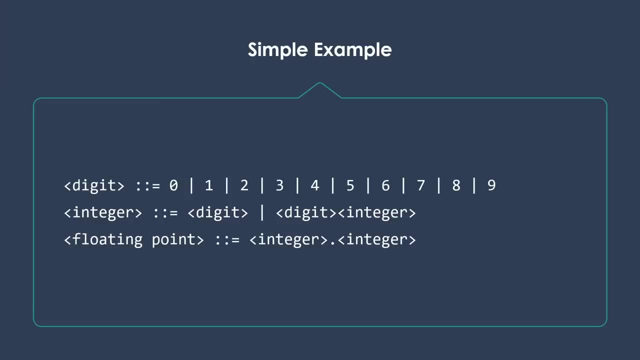 is to it. So BNF is very, very simple in terms of its structure. So a couple of examples I'm going to go through here. First of all, a fairly simple example where I'm just trying to interpret a number, see if it's a valid number, So I might have digit, and then it's zero, or one or two, or 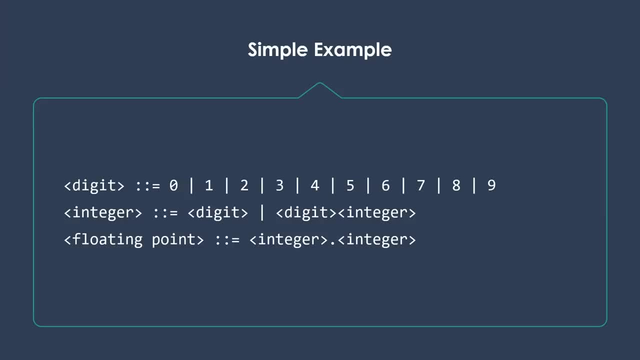 three or four or five or six or seven or eight or nine, Then I might represent an integer as being a digit, because it could be just one digit or a digit followed by an integer which will consist of one or more digits. Grammars in general tend to be inherently recursive. This is true of our 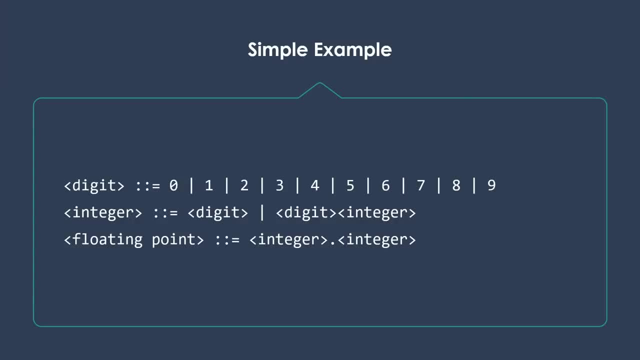 natural language grammars as well as our programming language grammars. Then finally, I have here floating point: goes to integer dot integer. Of course, when we think about the semantics of that that may not make sense to us, but that will parse correctly for. 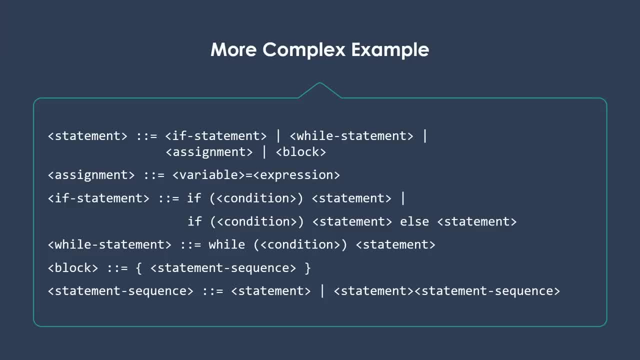 a floating point number in this form. Here I have a somewhat more complex though certainly incomplete example. This might be a fragment of a grammar for a C-based language like C or Java or C++, C, sharp, et cetera. So I have statement and I've provided four of the possible translations. 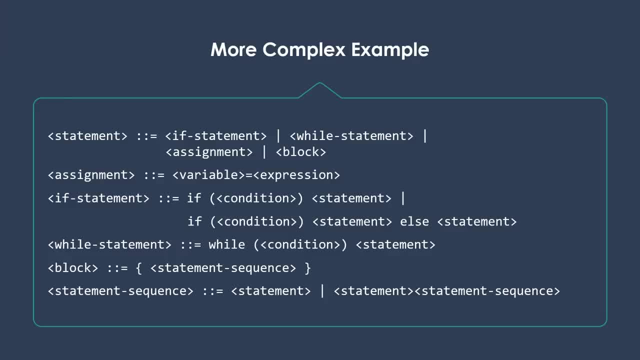 of statement- There are, of course, many more in all of those languages: An if statement. it could be a while statement, or it could be an assignment, or it could be a block. An assignment typically does look something like variable, though there are some other options besides variable, of course, and then the equal. 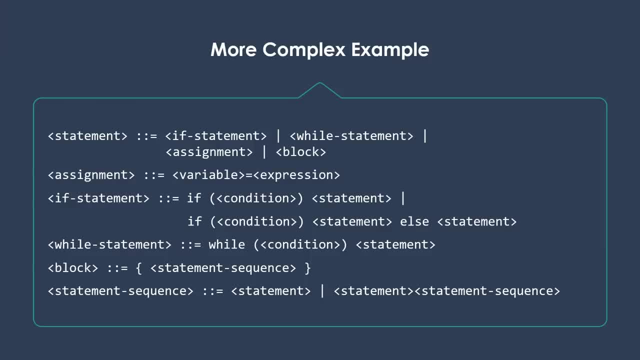 symbol and then some sort of expression. An if statement can be an if open parenthesis condition, close parenthesis and a statement, Or it might be if open parenthesis condition, close parenthesis statement, else statement, A while statement, of course. 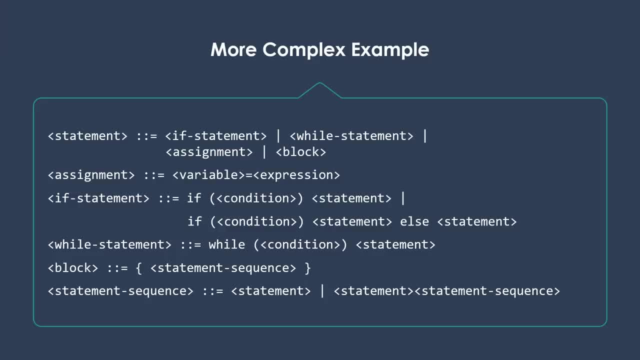 would be a while. open parenthesis condition. close parenthesis statement. A block would be: open curly braces: a statement sequence. close curly braces where a statement sequence is going to be a single statement or a statement followed by a statement sequence. So this would be a 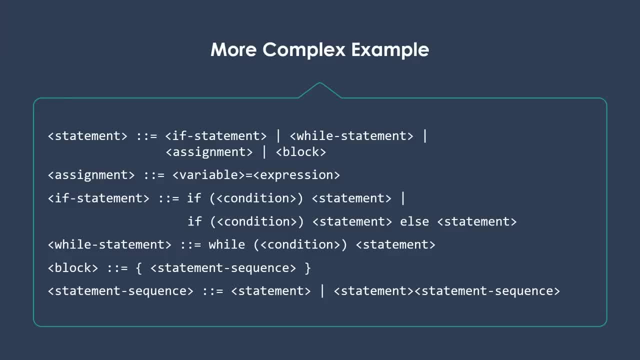 fragment of the grammar for one of those C-based languages. So I have a statement, a block and a statement sequence for both C-based languages. Now, of course, here I haven't gotten down to the level of terminals very much. I do have the equal sign and the parentheses, and 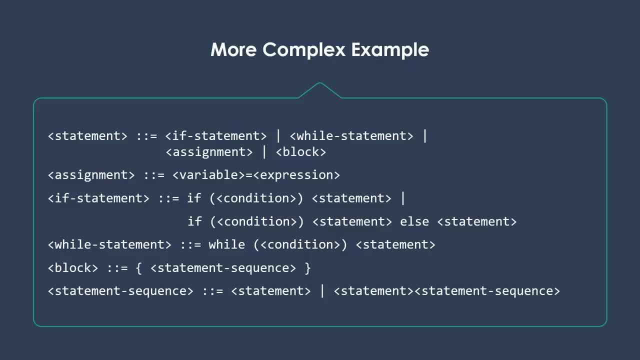 the curly braces, as well as the if and while keywords. But I haven't really addressed the identifiers and so forth And part of that was simply didn't have a lot of space. But another reason is that we often don't want to try to deal with those at the same time. We have both. 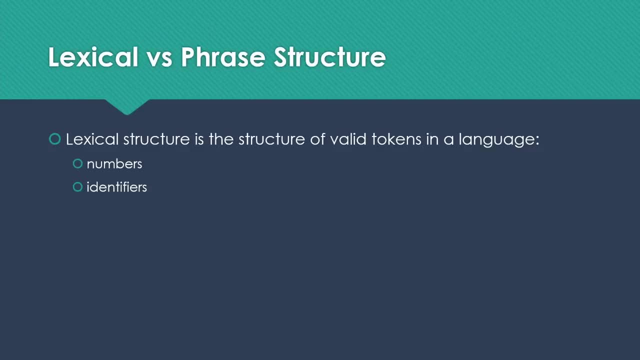 different definitions and different ways of using them, And so we're going to use the same definition of the word structure. So by lexical structure, we mean the structure of the valid tokens in a language, things like numbers and identifiers. By phrase structure, we mean the. 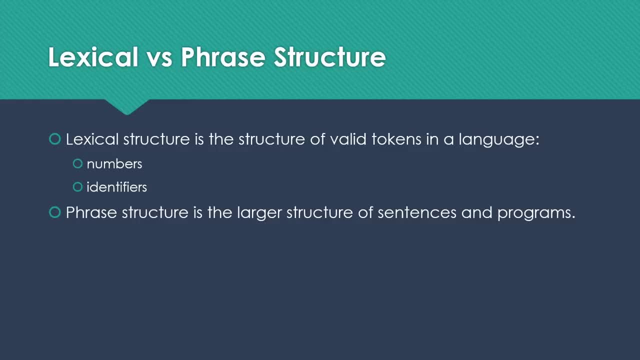 larger structure of sentences and programs, the kind of structure that the second example I showed you was about, whereas the first example was about lexical structure In general, when we're dealing with programming languages- and actually I don't know if you've heard of programming languages- 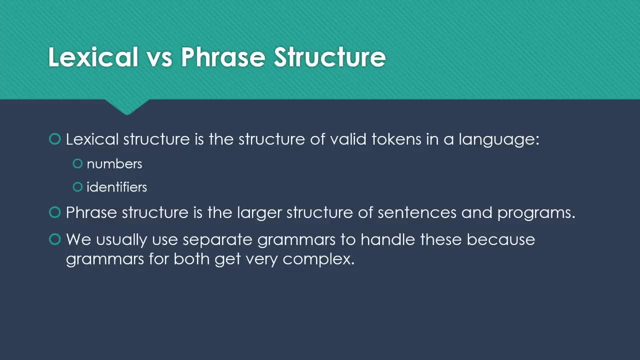 we tend to use separate grammars to handle lexical structure versus phrase structure Because when we try to combine them things can get very complex and ugly And in fact when we create compilers or interpreters for languages, those typically also usually handle what they call. 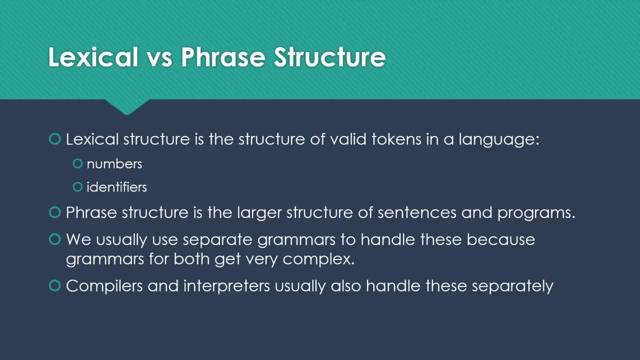 lexical analysis separately from going through the structure of the language and handling the phrase structure. So typically we do lexical analysis first, identify all these tokens and whether they're identifiers or numbers or keywords and so on, and then go through and apply the rules of a phrase structure for the language. 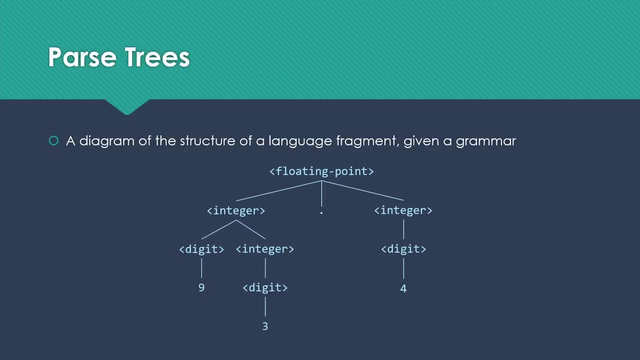 Before we end this video, I do want to talk to you just a second about parse trees and show you what those are about. The idea of a parse tree is that it's a way to demonstrate how a fragment of a language is structured, given a grammar. So here I've got the parse tree for the 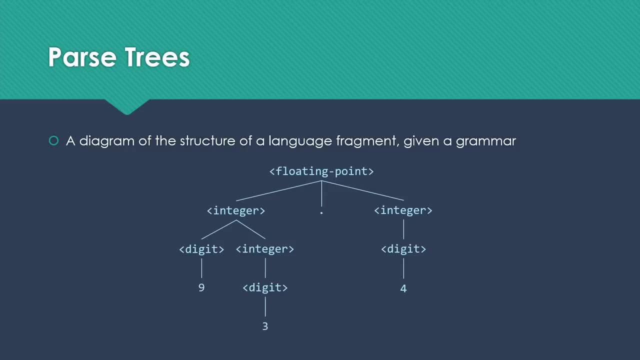 first example grammar that I showed as applied to the number 93.4.. That's a floating point, So it's going to consist of an integer- the string of digits- followed by a period, followed by another integer string of digits, And the integer, in the first case, will consist of a digit followed by a. 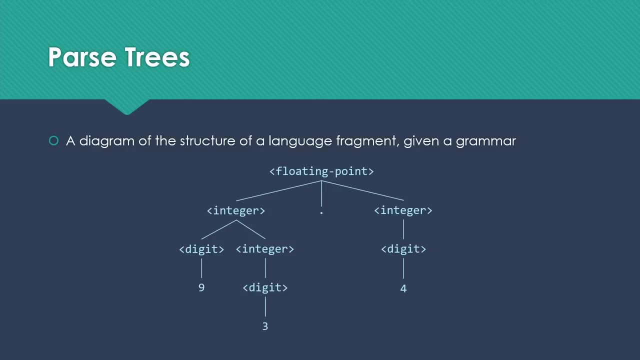 an integer, so we've got two numbers there. the digit will get translated into the nine for 93.4. the second integer will be just a single digit will get translated into the three. of course, the point we picked up with the overall structure at the beginning and the last part of the floating 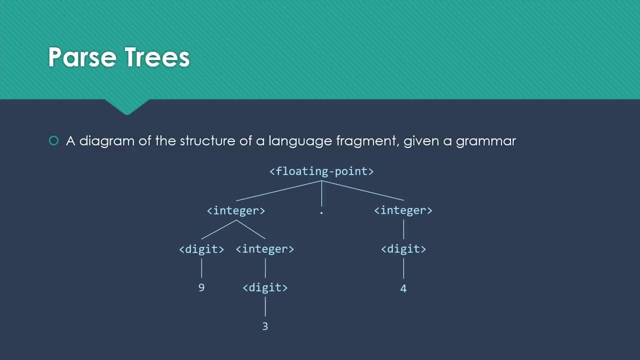 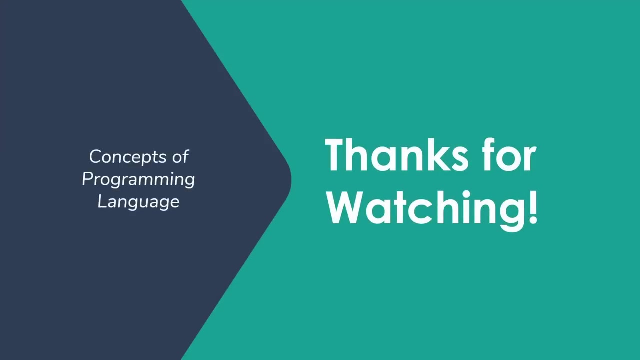 point. integer is just a single digit, which is, of course, four, so this shows us how that grammar structures that particular number. this will be very useful to us as we go on in the next video to start talking about semantics and ambiguity. thanks for watching. hope to see you next time when we will be talking about